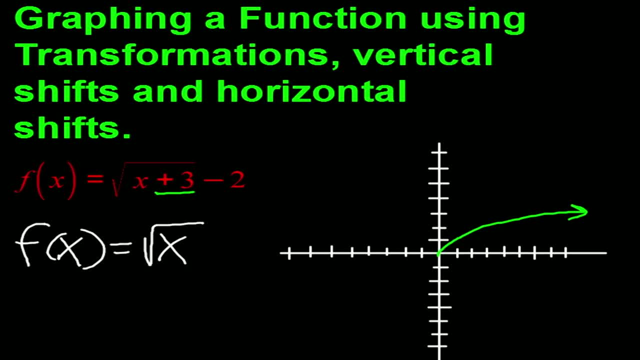 square root And any time it's inside the square root, or if it's a squared function or a cubed function or whatever it is- if it's inside, then that transformation or that shift is going to be horizontal. It's going to shift the function horizontally left and right. 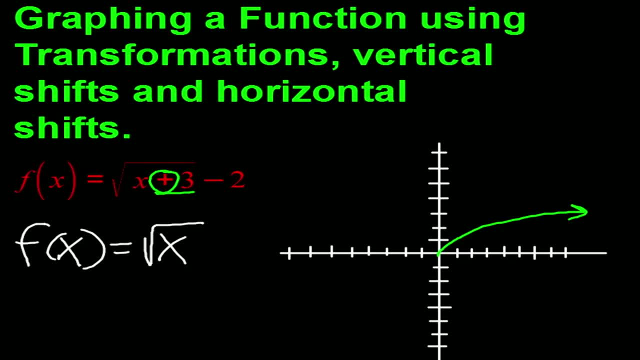 Now, normally we would think that a plus would shift it right, But it actually, when it's inside the function, it's opposite of what we think. So instead of shifting it right three places, it's actually going to shift it left three places to here. And so then, 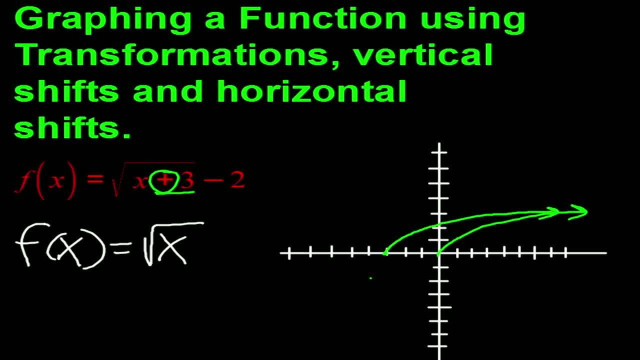 if I sketch it, it's still going to kind of go this way like that, Alright. And then I go and I focus on the outside of the part of the function, the minus 2.. And when I go outside the function, what that does is it shifts it vertically up and down And it acts exactly. 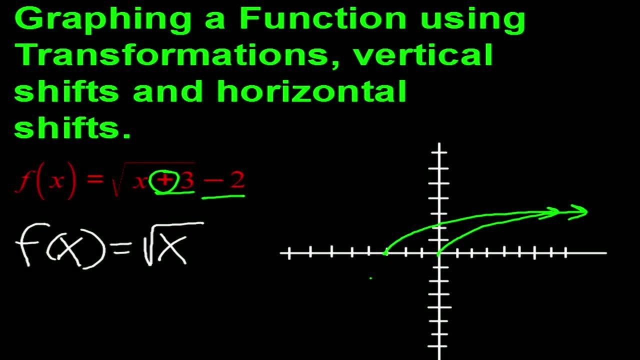 the way we would expect it to act. If it's negative, it's going to shift it down. If it's positive, it's going to shift it up. In this case, it's a minus 2.. So we start here and it's going to shift it up. So we start here and it's going to shift it up. 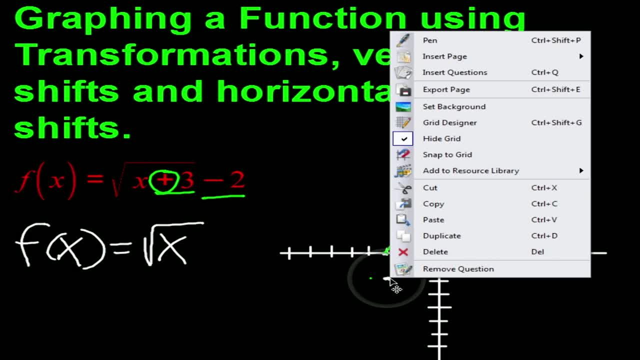 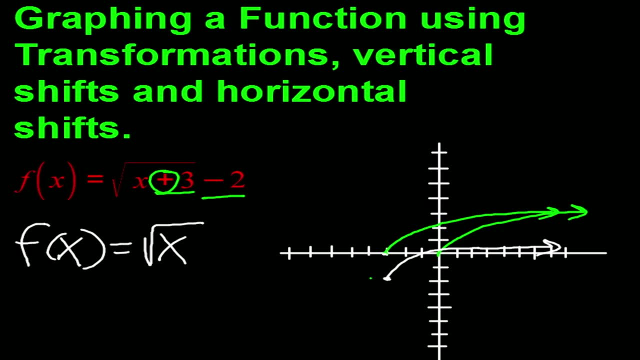 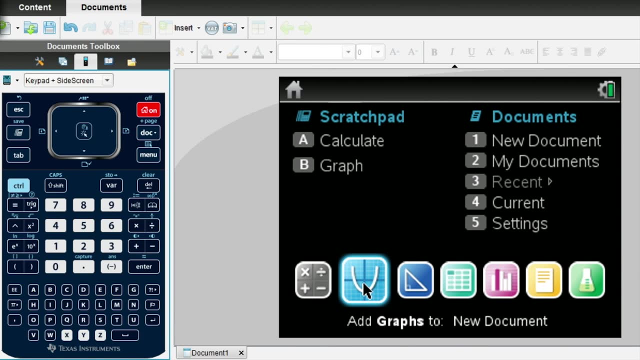 And it's going to shift it down minus 2.. So actually our graph is going to start here And it's going to go kind of like that. Now I'm going to verify this with the TI-NSPIRE calculator to kind of give you an idea of exactly what I'm talking about And to give 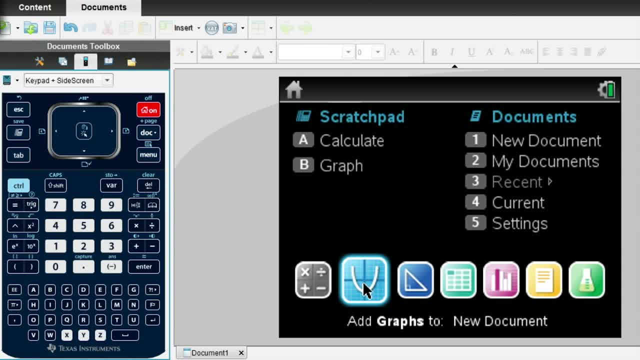 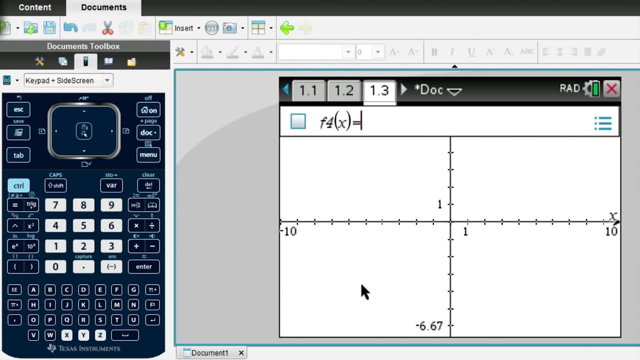 you a little bit of help with the INSPIRE itself. So first of all I'll start off with the graph page And then I'm going to type my equation in. So I'll do the Control key to get to the Square root function And I'm going to type: 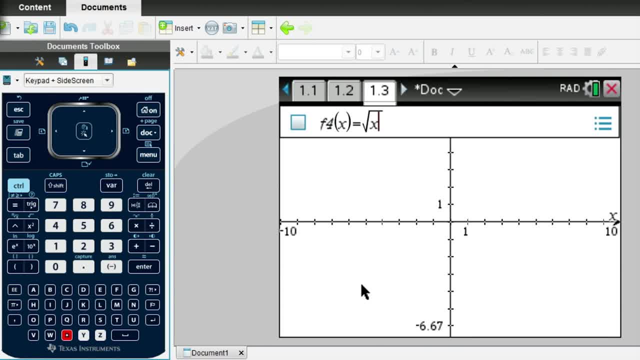 in X plus 3.. And then I'm going to use the right arrow key up here. That takes me outside the square root And I do minus 2. And if I press Enter, that graphs it And notice that basically is the same position on the graph as what I just manually graphed and 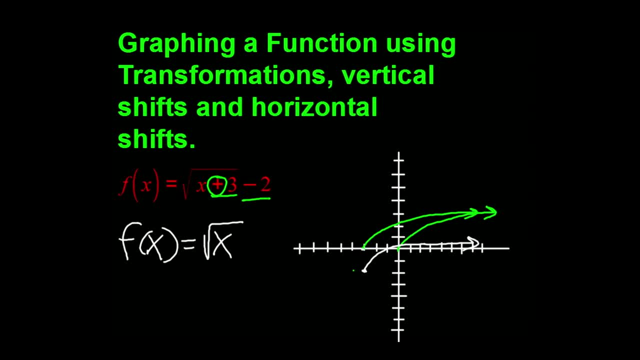 graph over here on my page. this function right here, so I just verified how these shifts work. the inside shifts at left and right, the outside shifts it vertically.